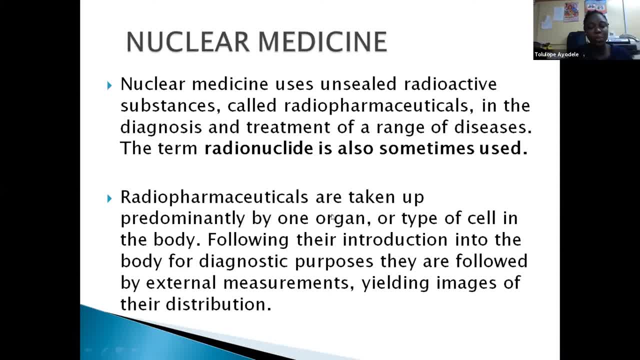 or taken orally, and so once the patient has taken up these radiopharmaceuticals, they are distributed throughout um the body. so, following their introduction into the body for diagnostic purposes, they are followed by external measurements or radiation detectors, whereby we could um, actually um, because we could actually image the um body and know the particular. we know the particular. 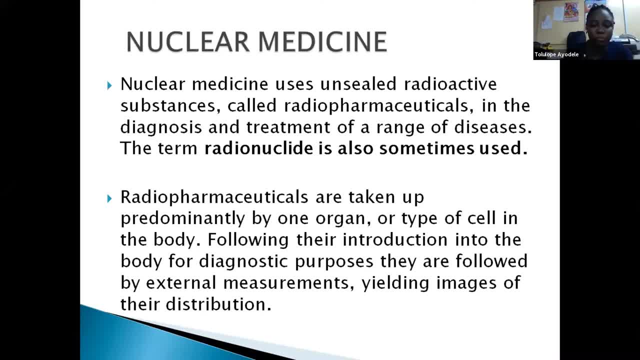 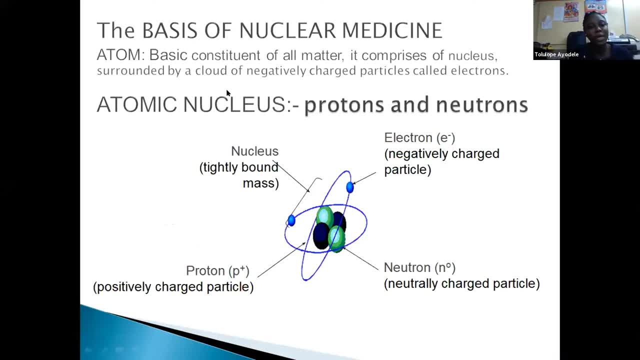 um organs to be imaged. so let's look at the um basic um constituents of atom. we all know that atom is the basic um constituents of matter. it's comprises of nucleus- from our basic understanding of um physics- and it's surrounded by electrons- negatively charged electrons. we have the understanding. 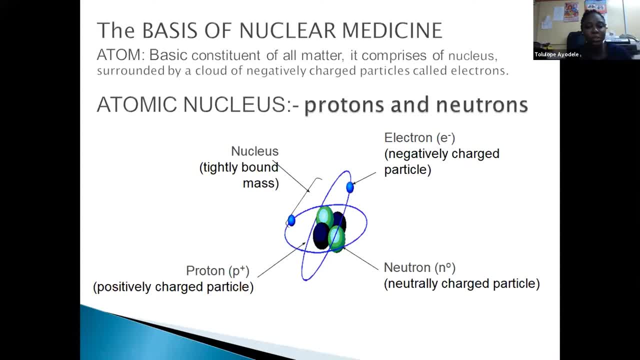 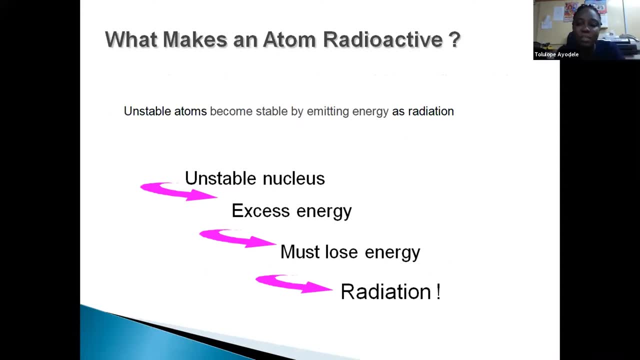 that it has the protons and the neutrons. so what makes an atom radioactive? we talked about um using unsealed radioactive sources and um for radiopharmaceuticals, whereby we combine radiation and the drug. so the radiation is actually labeled with um, this drug. so where? 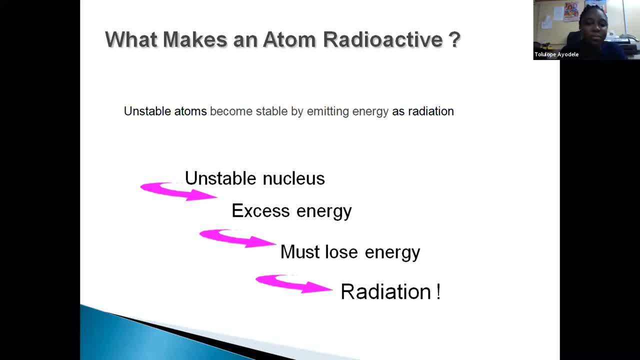 we what we do? we mean by an atom being radioactive. we have an unstable nucleus. for an atom to be radioactive, it starts to be unstable in the sense that it has an equal number of protons and neutrons. either the neutrons is too much or the protons is too much so in order to be um and it's. 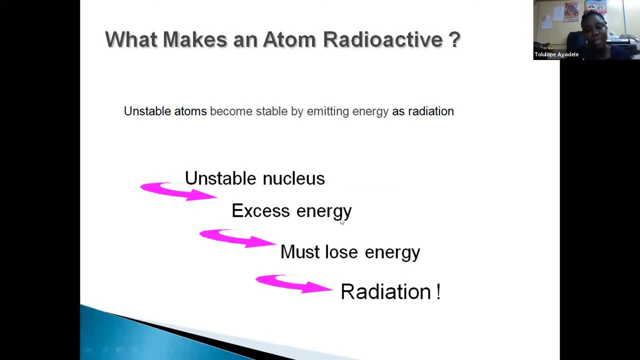 it has a lot of um excess energy. so in order to read off this um energy, it loses of this energy in the form of radiation. it could be in the form of a particulate radiation or electromagnetic radiation. so let's we briefly look at the different types of 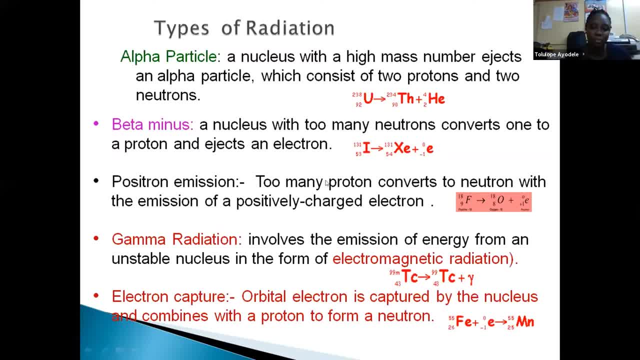 ionizing radiation. normally we use ionizing radiation in nuclear medicine because of the circuit, the neural properties, that they have sufficient energy to actually um cause um ionization. but there is not all the types of radiation that we use. we go through that during the course of the lecture. we have the alpha particle, which has the high mass number and from 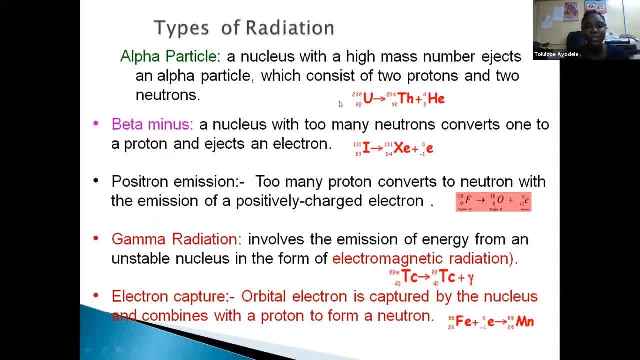 as you can see from my screen. you can see that you have the basic knowledge of one and half a particle is. it's a. it's a heavy as an heavy element. an example is uranium-238, and this is an example of a nucleus that undergoes an alpha particle as its mass number decreased by four. 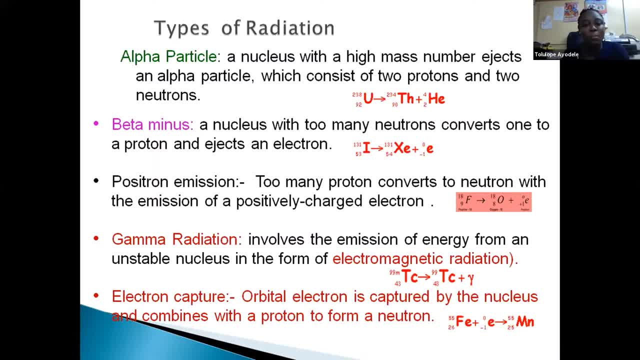 emission of an helium particle, while the atomic number reduces by two. so for the beta minus particle, we have a nucleus that has too many neutrons and with a bit to convert, with a bit to uh, it's converting the neutron to a proton as a result of the excess number of nutrients. 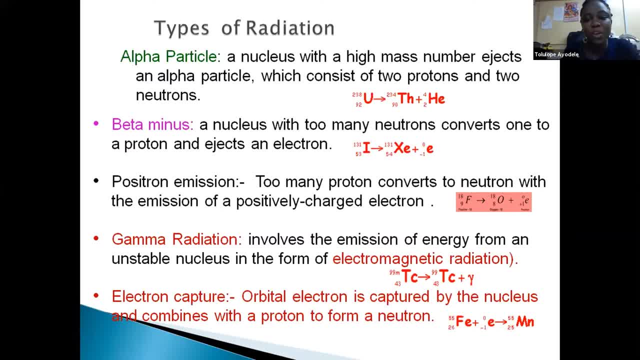 so an example of um, irradionuclides or radiation, a radioactive element that only goes beta minus, is iodine 131, while that's urban positron. we have another type of radioactive decay: decay with positron emission. an example of um, a radioactive element that only goes with position emission, is fluorine 18.. 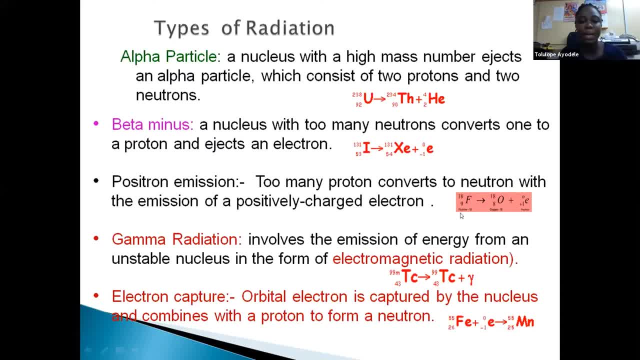 this is one of the um radio isotope we use in nuclear medicine for radionuclides, So it has too many protons and combative neutrons, whereby emitting a positively charged electron or a positron. We have the gamma radiation, which involves the emission of energy from an unstable nucleus in the form of electromagnetic radiation. 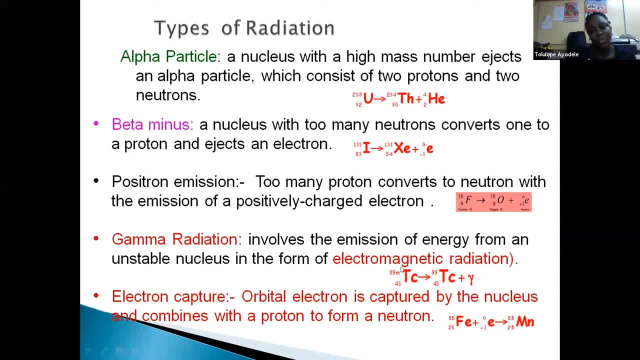 Note. the electromagnetic radiation we use in nuclear medicine is the gamma ray. Because it has a long penetrating power, it can be easily imaged And one of the radionuclides that emits this gamma radiation is technician 99M. The M is a metastable light. 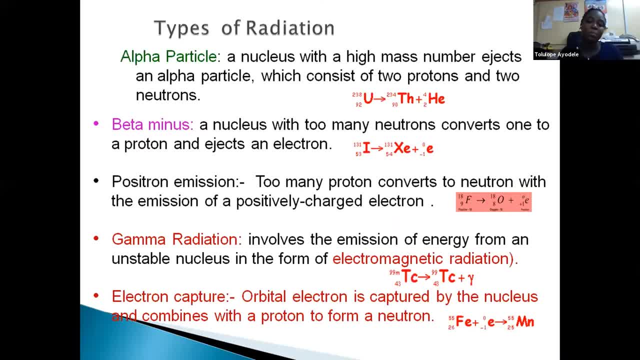 It has a considerable life span. It exists in matter for a period of time before it actually decays into technician 99, thereby emitting gamma radiation. So the technician 99M is the most widely used radionuclide in nuclear medicine, for radionuclide imaging. 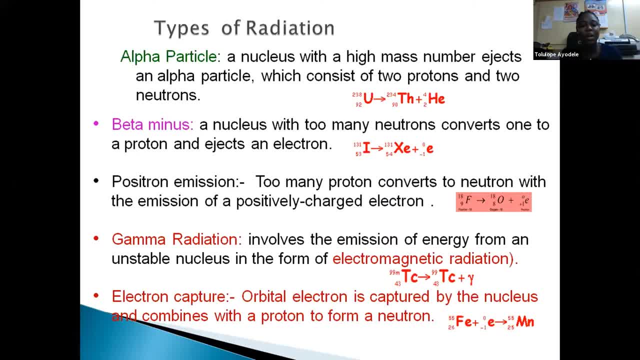 It could be labeled with a variety of radiopharmaceuticals, depending on which organ to be imaged Next slide. So we have the. We also have the electron capture, whereby an orbital electron is captured by the nucleus and combined with a proton to form a 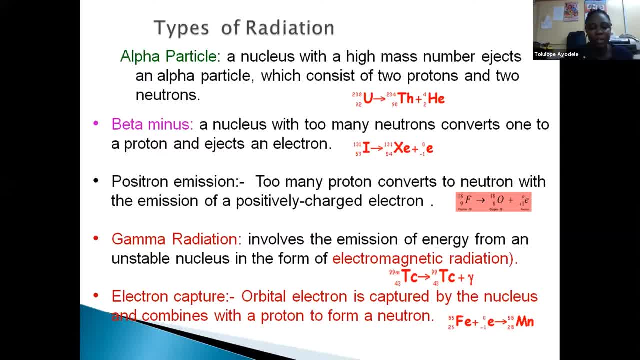 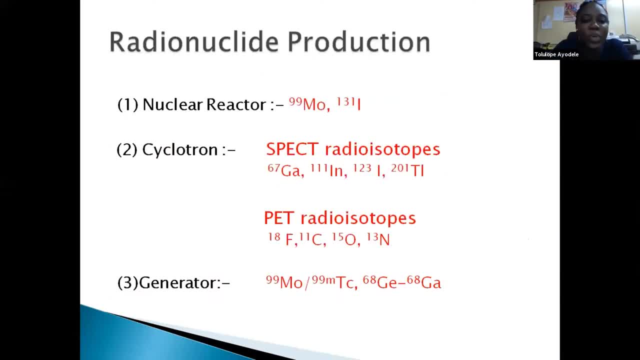 neutron. So an example of a nuclear that undergoes electron capture is the ion 55.. Let's look at the various types of production of this radionuclide. Where can we get these radionuclides from? We have the nuclear reactor and examples of these radionuclides. 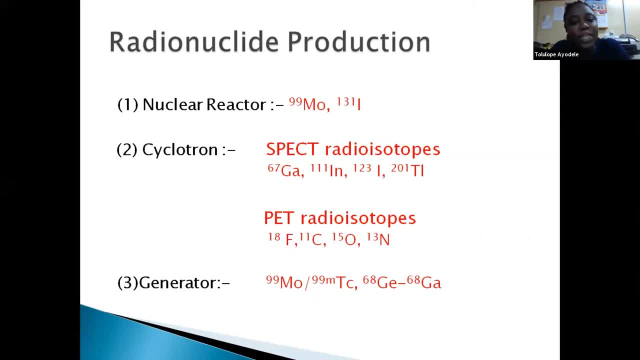 that are produced from the nuclear reactor includes the molybdenum-99.. This is the parent radionuclide for the technician-99m, So the technician-99m is actually separated from the molybdenum-99m. 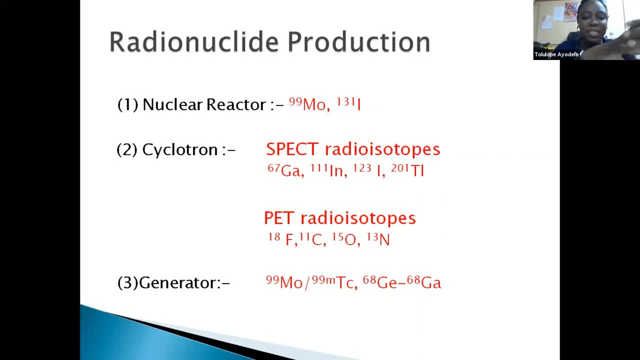 We also have the cyclotron, whereby spects with the isotopes are produced. These include the gallium indium, as you can see from the slides For the pet's radioisotopes. let me make it clear that the spects, radioisotopes, emit gamma rays, So we could actually image. 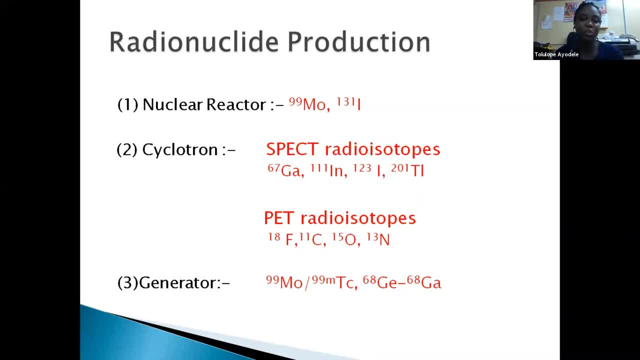 with the spects, spects with the spects single photon emission, commutator tomography system. So we talk about that in the course of the presentation. And we also have the positron emitting radionuclides, whereby the pet system. we could use this, the pet system, to image. 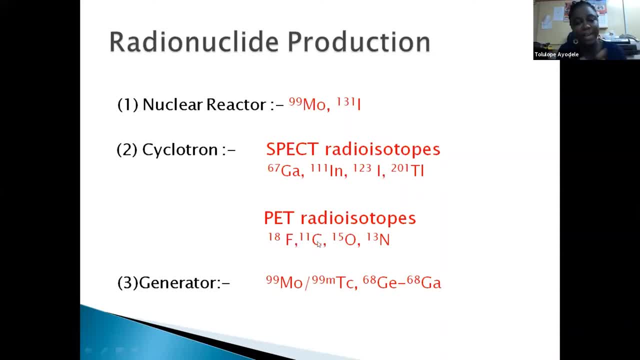 the radionuclides that emit positrons. An example of some of these radionuclides include the fluorine-18, carbon-11, oxygen-15 and nitrogen-13.. So there's the system of the generator, whereby we have 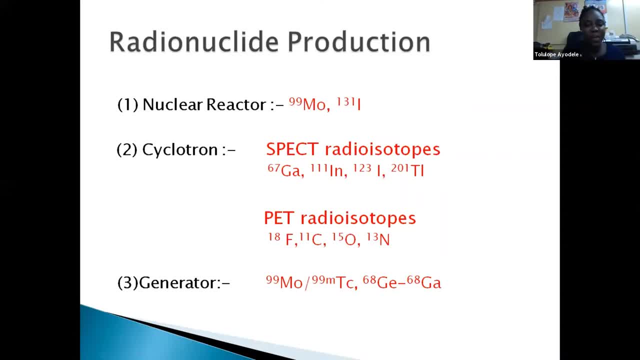 a parent-daughter generator. The parent-daughter generator- an example of the parent-daughter generator- is the molybdenum-99, technician-99m generator, whereby we're able to separate the daughter radionuclide. The daughter radionuclide is the technician-99m 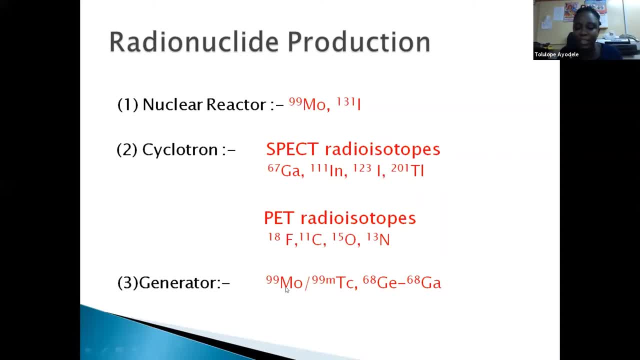 and while we're able to separate the daughter radionuclide is the technician-99m, the mother radionuclide is the molybdenum-99.. So we're able to separate it from the mother radionuclide through a chemical process And one of these, as I said earlier, the Technician. 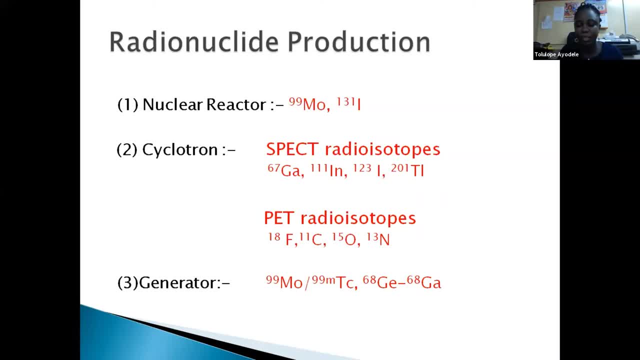 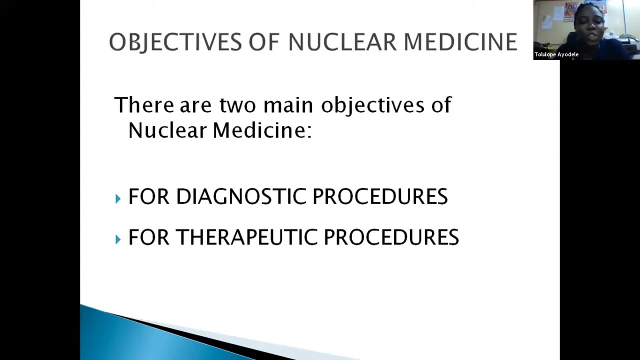 99M is the most widely used radionuclide in nuclear medicine or radionuclide imaging. So we also have another example of the generator produced radionuclide, which is the germanium-68, gallium-68.. Nuclear medicine has two objectives, So it's used for diagnostic. 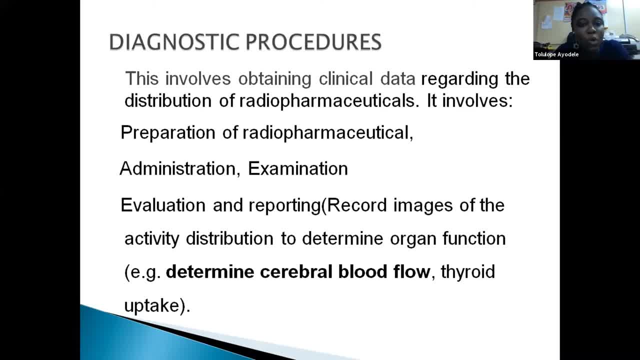 purposes and therapeutic purposes. So it involves a situation whereby once the radionuclide has been administered, once it's injected into the body of a patient intravenously, or it's been swallowed by taking orally, made via the capsule. So we could 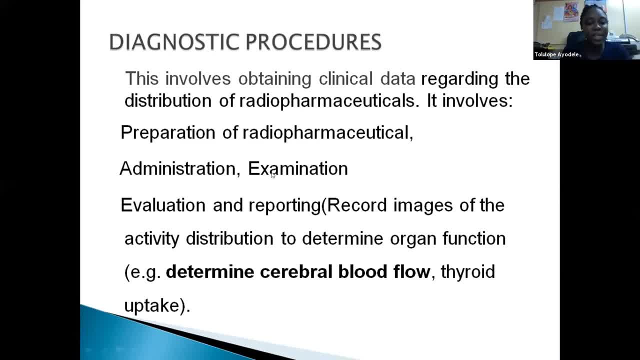 inject radionuclide into the body of a patient intravenously or it's been swallowed by taking orally, made via the capsule. actually, um, our site has been administered. it involves the process by whereby the patient is examined and evaluated and, of course, the records of the images of the activity distribution. 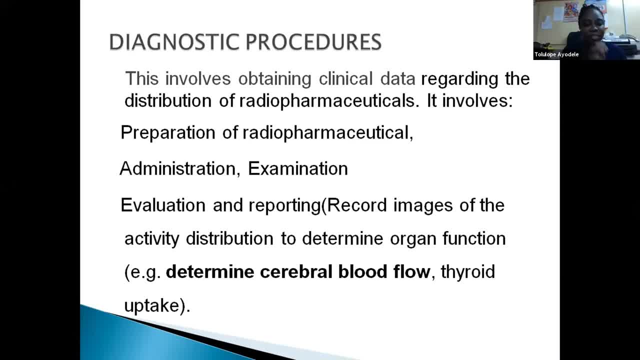 can be seen in um, the radiation detector. so for the purpose of diagnosis, and some of the applications involve organ function, nuclear medicine is a functional imaging modality, as compared to radiographic images, whereby anatomical information could be um deduced. so you could actually know how well an organ is functioning through a nuclear medicine or procedure. so 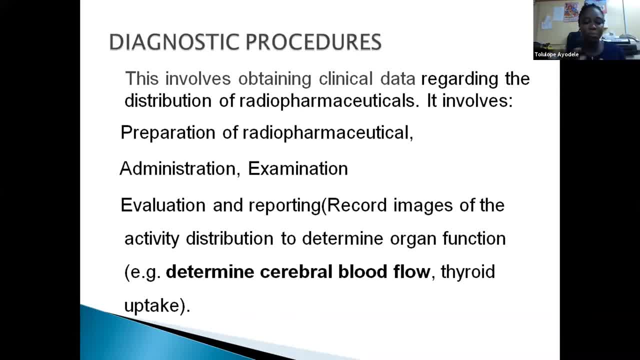 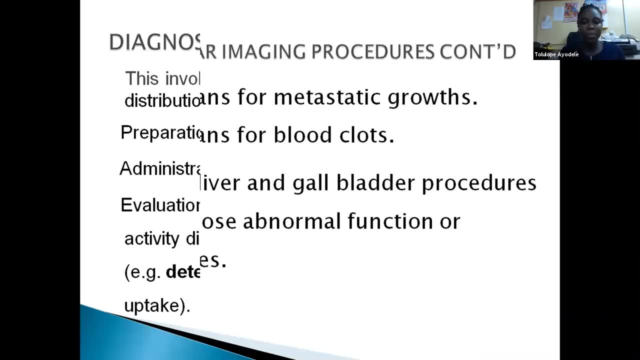 examples of some of these, um, of some of these functions include: you could determine the blood flow, the race at which, uh, the blood is flowing in the brain, the rate at which, um, the thyroid is taking up iodine, and many more, um many more functions. other examples include bone scan, whereby you could detect bone tumors, the extent of metastasis. 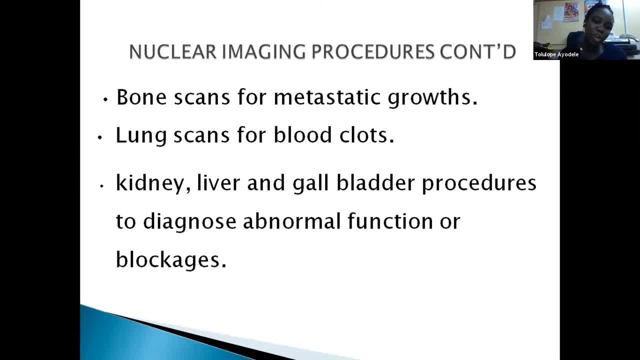 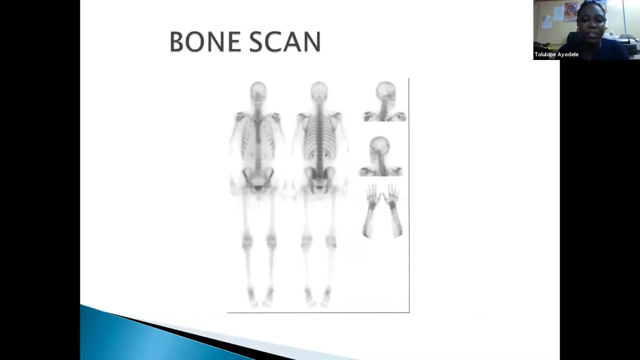 lung scan. you could actually detect blood clots via a lung scan and, of course, in kidney, liver or blood you could actually you could also determine or detect abnormal uh functions or blockages. so this is a typical example of a nuclear medicine scan, a bone scan, whereby you could actually- um, it could actually depict. 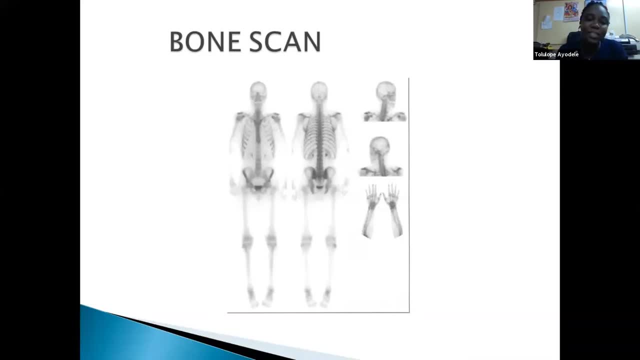 depict the um. the bone meta metastasis could actually detect some bone metastasis, indications of bone metastasis, metastasis, arthritis and even infection- bone infections, okay, from a nuclear medicine. so this is a typical example of a bone scan and the radiopharmaceutical that is used. 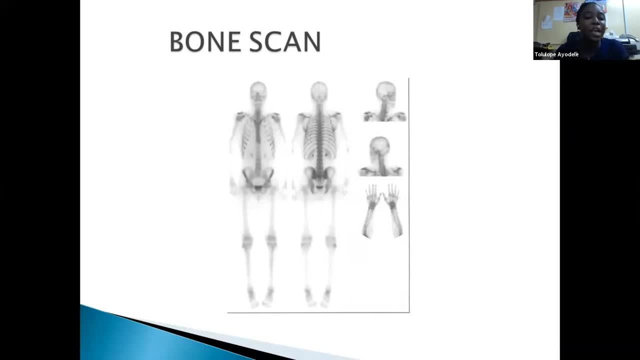 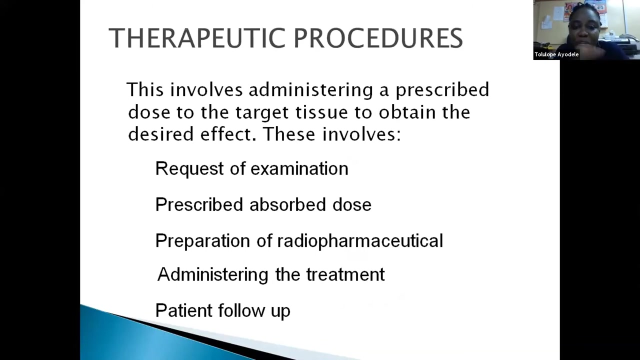 yes, an example is technician 99m, mdp or hmdp. so we have: the mdp is the drug that has affinity for the bone and is actually actually labeled with the technician 99m that emits gamma rays. so nuclear medicine also has this therapeutic purpose, not only used for. 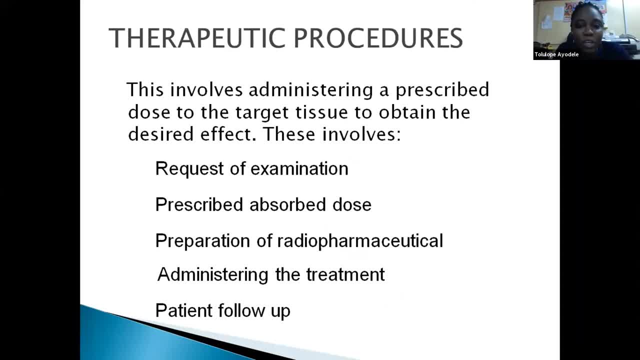 diagnostic purposes. so let's take a look at some of the procedures of a therapeutic procedure. first of all we have the requests for an examination. there's a prescribed dose and um. the preparation is actually of the radio, is actually done by radiopharmacists. requirements is an interdisciplinary of field that consists of the very numbers of um professionals. 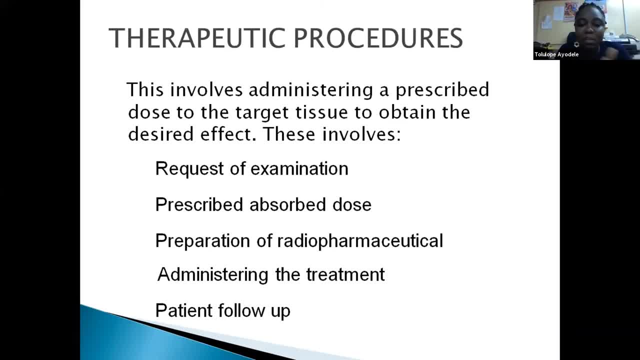 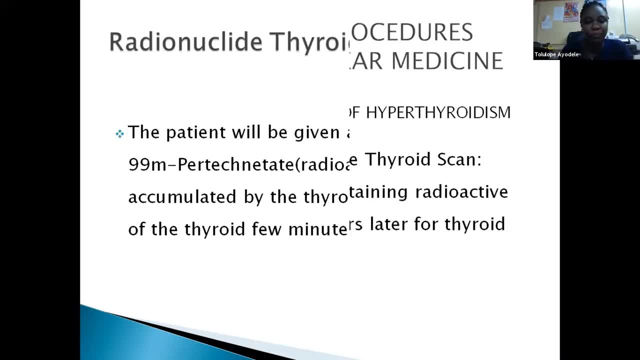 so we have. then, once it has been done, we can then go to the next slide. so here we will. I've got the first step. we're going to be doing, uh, the road test. um, the first step is that you should have a pre-treatment or your pre-treatment. 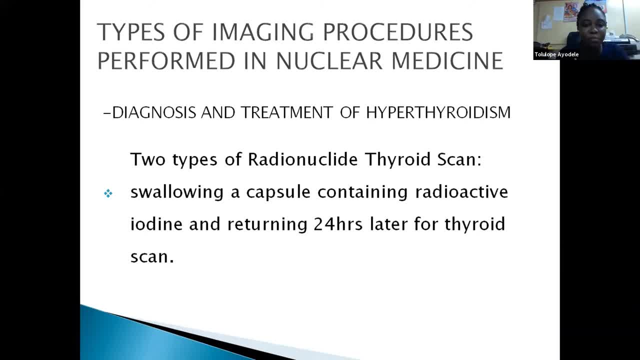 so here we will go to pre-treatment, which we have been working on to get this to be a pre-treatment, um. this is a pre-treatment, so we're going to have a pre-treatment so that the patient can do a pre-treatment, um. the second is that you are going to have a telemedicine. 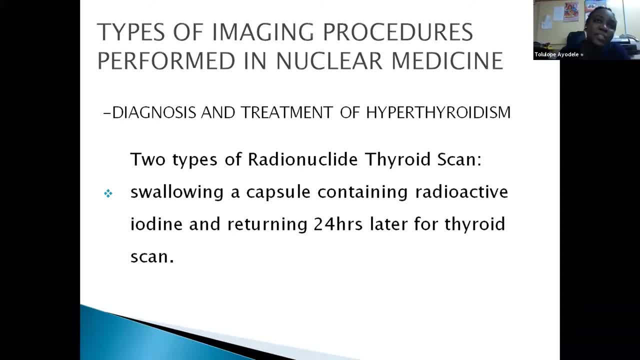 uh, that you are going to be using just to use for�itp, and this is a well-known technique which we- hypothyroidism, thyroid cancer- and you could actually the patient could be actually offered a nuclear medicine scan for the diagnosis and the treatment of the thyroid disease. 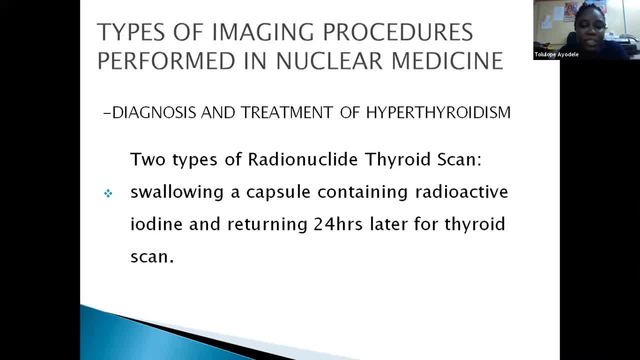 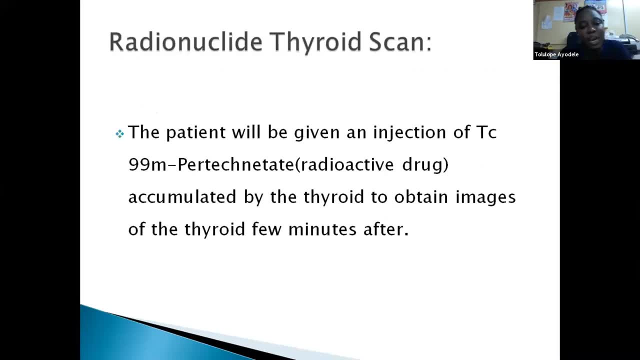 by swallowing up a capsule, a solid, you know, a capsule of iodine-131, okay, and returning 24 hours later for the thyroid scan. The technician might deny him pateknetase-2 could be used for the thyroid scan, okay. 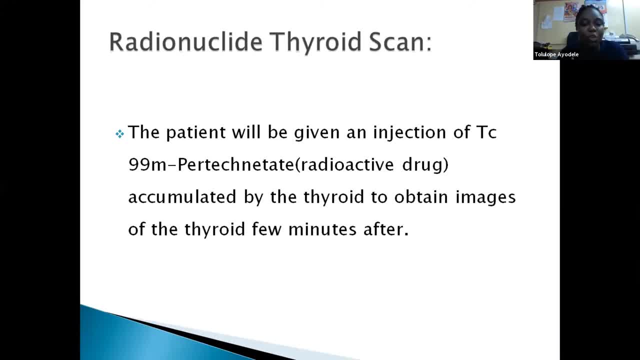 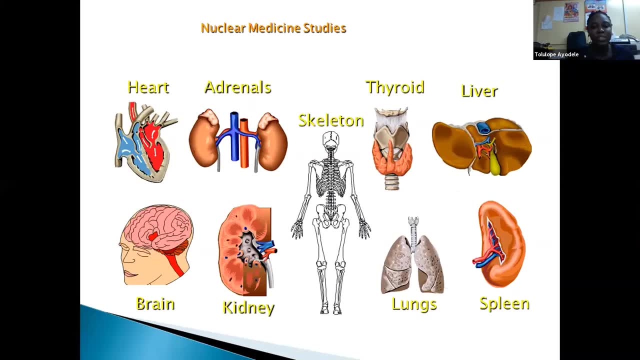 So once it's accumulated in the thyroid, we could obtain images of the thyroid few minutes later. So here's a typical illustration of what we can use nuclear medicine to do. So nuclear medicine can be used to image the heart, the adrenals, the skeleton, the thyroid. 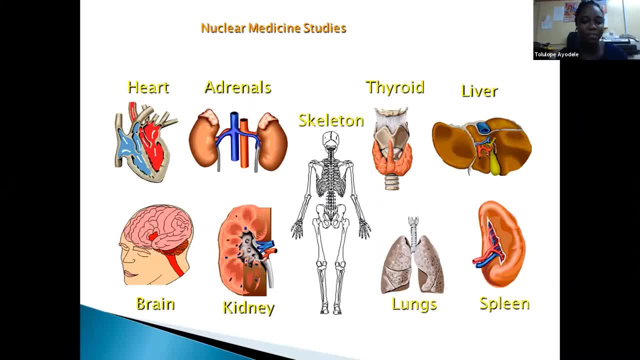 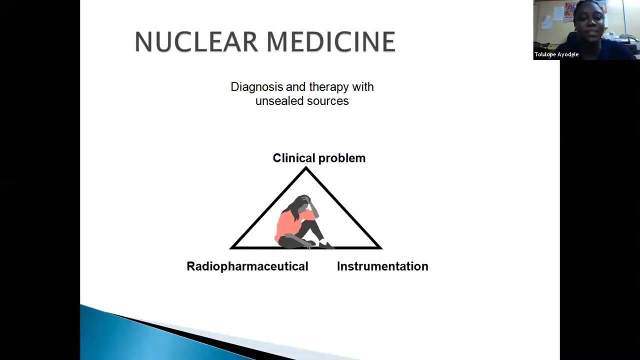 the lift is a bit head length We have you can use to image the brain and also detect the function or any detect any abnormalities that is, inside any of these organs. In essence, this is a summary of what nuclear medicine is about: an education for a problem. 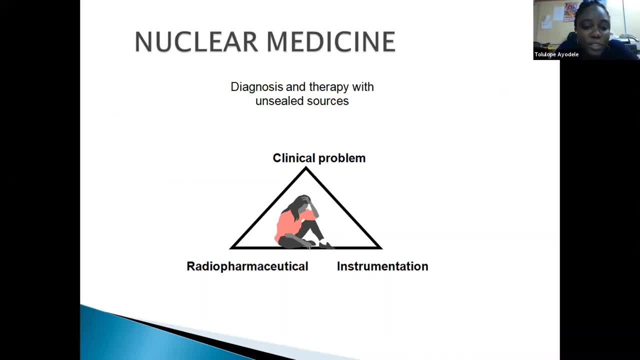 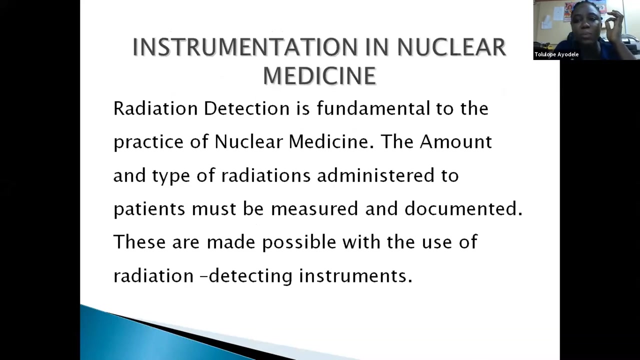 And we use an ayuda source of San Jose pharmaceutical. Once it has been injected, swallowed, is detected by slides. so we have. so let's talk about the instrumentation in nuclear medicine. i hope you can all hear me. so radiation detection is fundamental to the practice of nuclear medicine. the amounts and the type of radiations administered to patients. 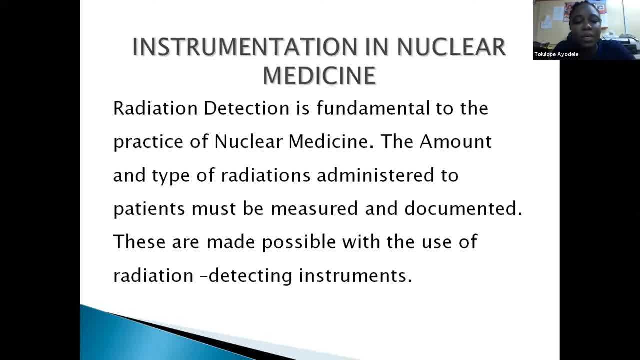 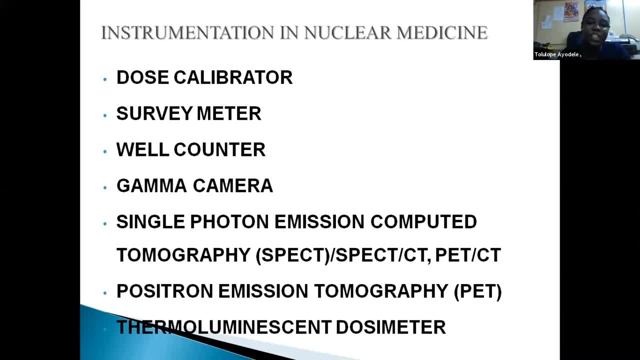 must be measured and documented, so these are made possible with radiation detecting instruments. here's the list of the um equipments or the detectors that we use in nuclear medicine. we have the dose calibrator, the survey meter and the procedure. there are lots of um, so we're 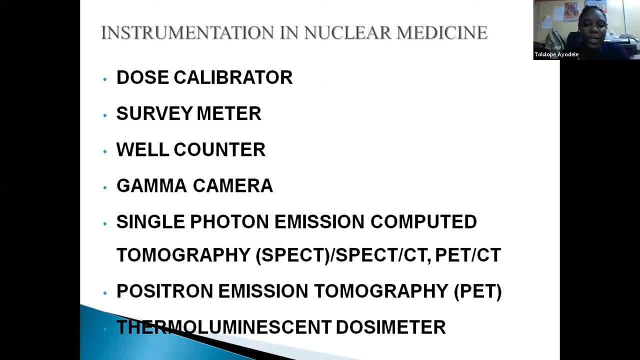 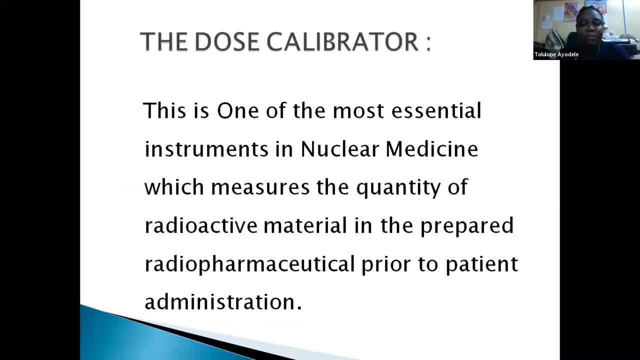 talking about. so we'll be talking about some of these um equipment. you'll be talking about some of these equipments and their functions. so we have the dose um calibrator, which is very essential, which is a very essential um equipment in nuclear medicine and it is used to measure the quantity of radioactive material in the prepared once the 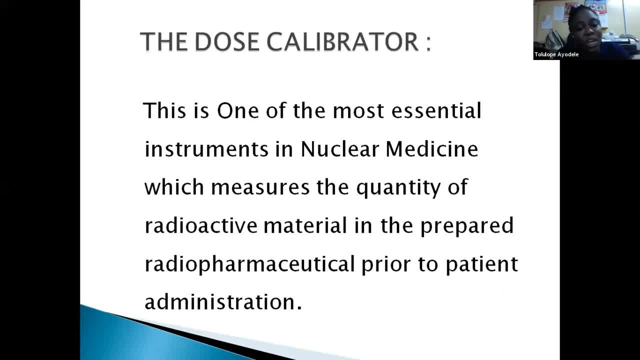 uh, the principle has been prepared. you could actually measure the um quantity, the activity in terms of uh, the amount of radioactivity in the material, um curie or um vikrel. so with depending on any um, on any radioactive substance you you want to um measure. it could be the. we can measure the um iodine one, three, one. 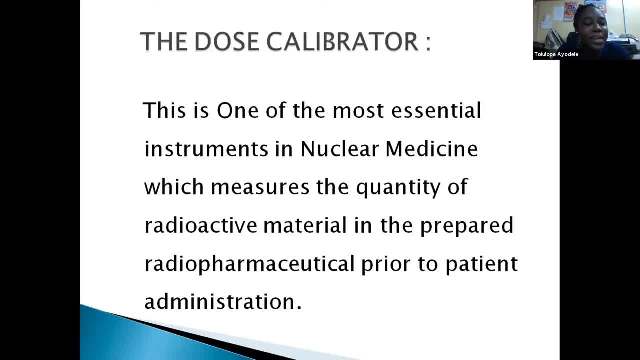 we could measure the technician 99m. any um, radio nuclide, radioactive substance could be measured with the dose calibrator and this is actually done in order to minimize um, to prevent or to avoid on the dosing. So this is done before being at. this is actually done. 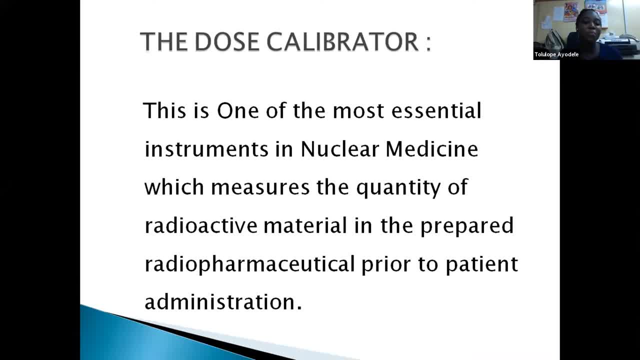 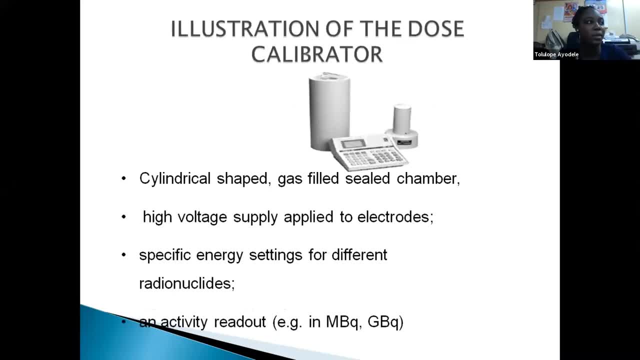 The adrenopamcica is actually measured before being administered to the patient. I hope you can all hear me. So this is a typical illustration of the dose calibrator and it has. it's a spherical shape and it's gas filled. 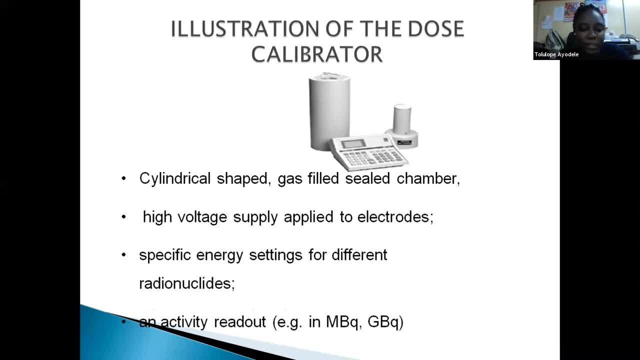 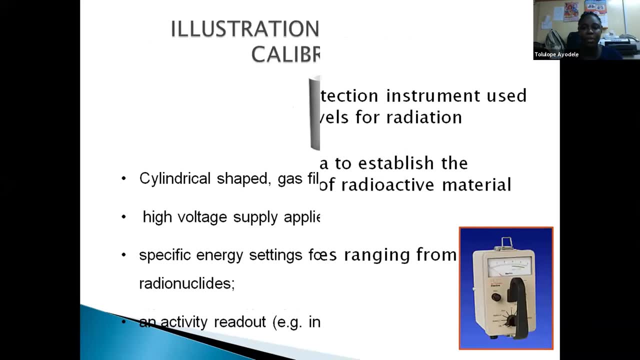 It has various components, as you can see, and it's actually with the activity in Becquerel, It could be that the megabecquerel or gigabecquerel. So let's look at the another instrument that is used in nuclear medicine. 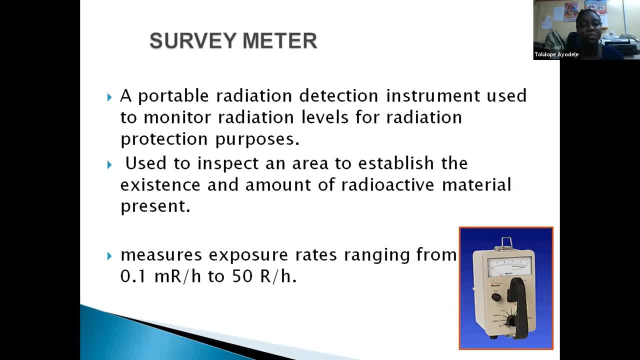 We have the survey meter, the possible radiation detector. It's handheld and it's used to monitor radiation levels for the purpose of radiation protection, So you could actually detect the level of radiation in an area, be it natural or in artificial radioactivity. 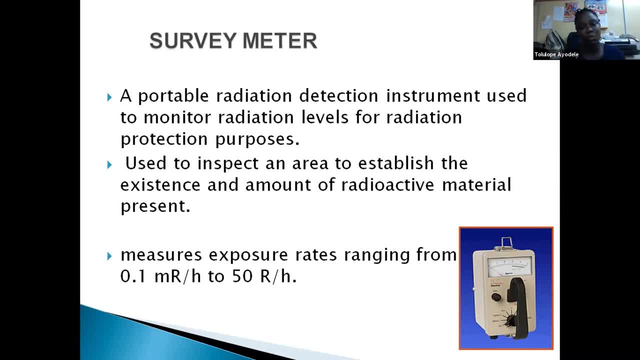 But we use artificial radioactivity in nuclear medicine. Actually, we do not use natural radioactivity. This is due to the fact that it has the natural radioactivity, has a very long lifetime and it doesn't have the inherent properties that we need. 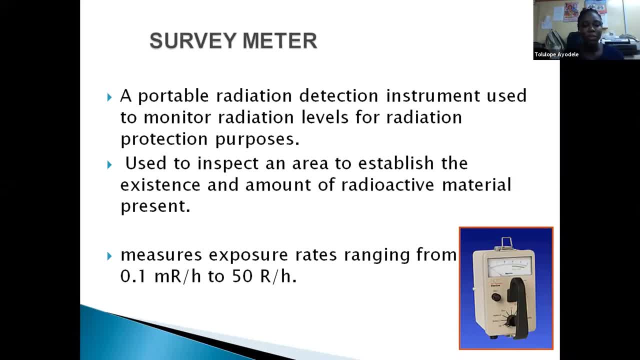 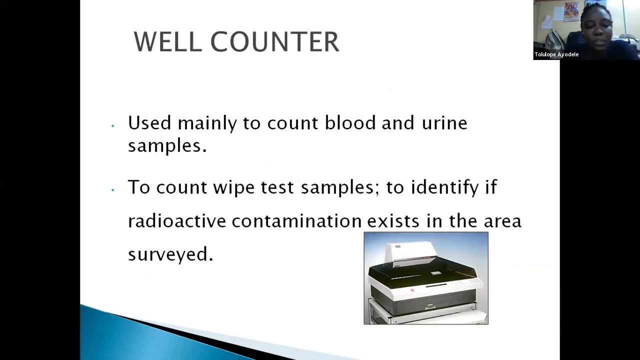 So for in radionuclide imaging. So it's measures in exposure rates of melleron gene And this is the range in 0.1 to 50.. We have the well counter as well, which is used to count blood and urine samples. 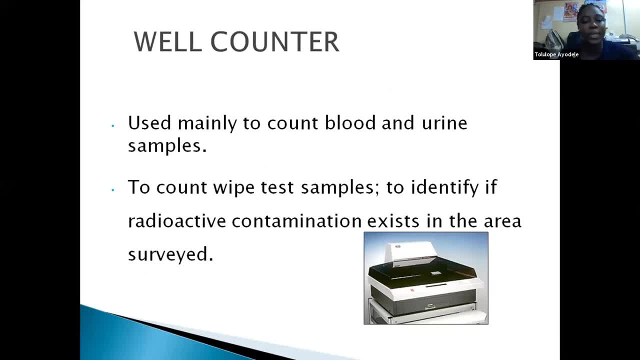 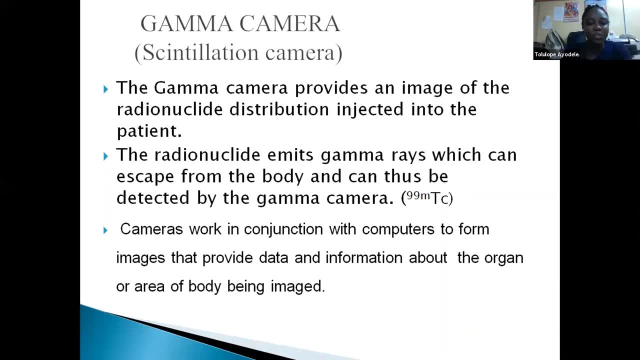 And it could identify radioactive contamination existence in the Soviet area. So we have the gamma camera as well. My time is running So I'll just skip through. We'll still get the presentation after. So we have the gamma camera, which is the most widely used equipment in nuclear medicine. 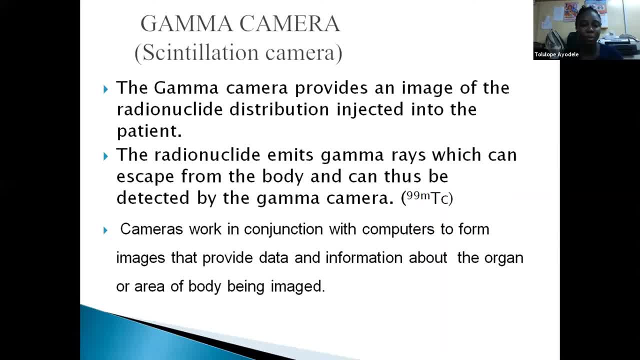 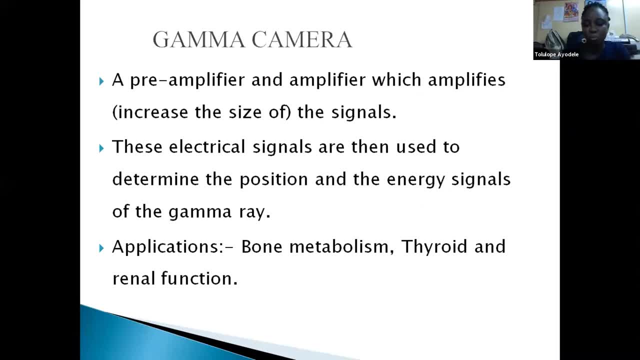 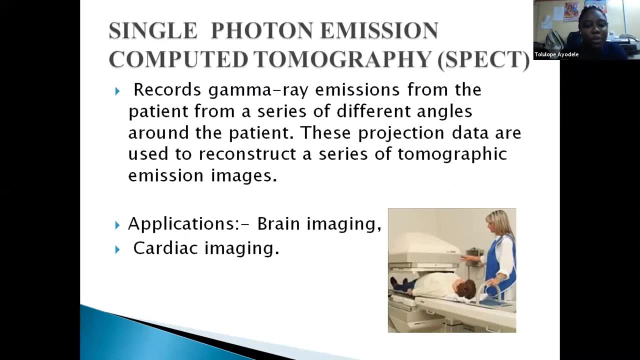 And it's used to image the radionuclide distribution in the patients. So this is a typical example of how the gamma camera looks like. We have the SPECSU, which records the gamma ray emissions from different Angles around the patients. 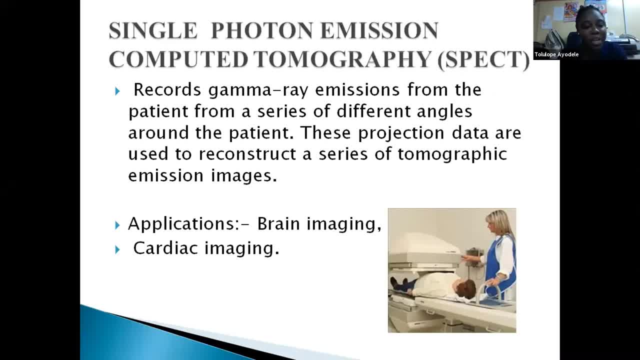 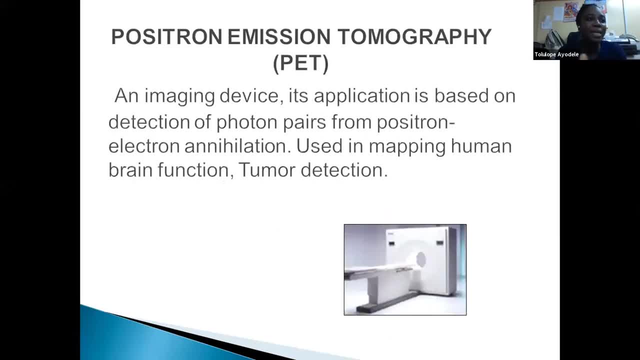 And the applications for this is in brain imaging, cardiac imagery. We use it to measure, to image the brain And also, of course, the ads, and to detect abnormalities in any of these organs. We also have the PETS, which is whereby we use a positron emitting radionuclide. 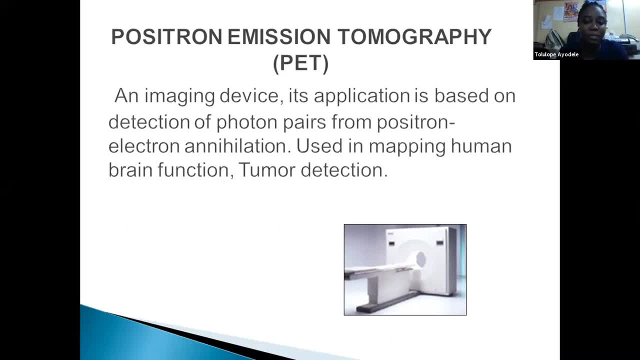 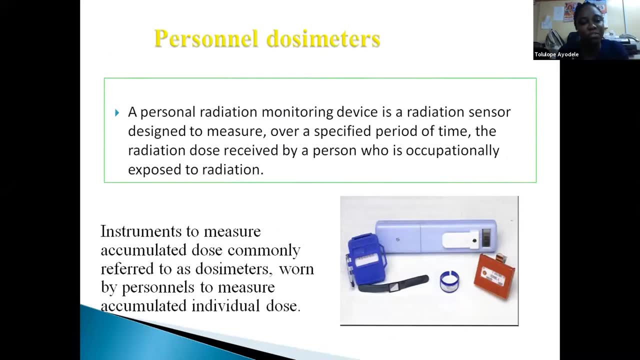 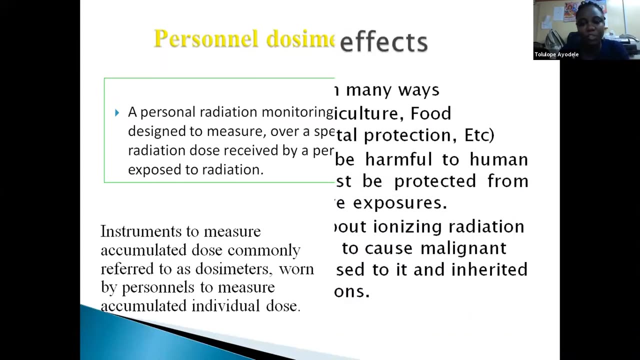 in for the diagnosis when we use the PETS scanner. So applications for this, we have the brain function, too much in brain function and too much detection. So the personnel with the data have been treated by the previous speakers. I'll just quickly run through. 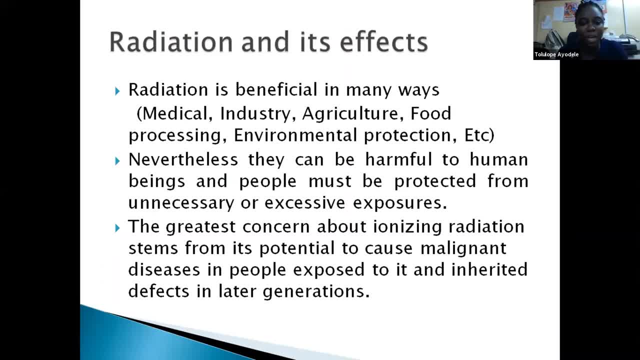 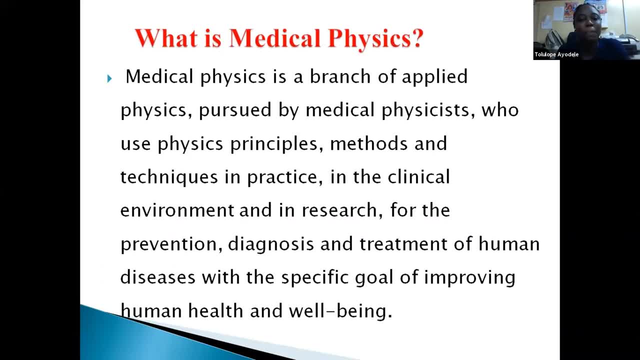 So the radiation has its effects, as the previous speakers have talked about. So, and we need to actually take notes of this. So what is medical physics? Medical physics has to do with. Medical physics has to do with. Medical physics has to do with with the application of physics. 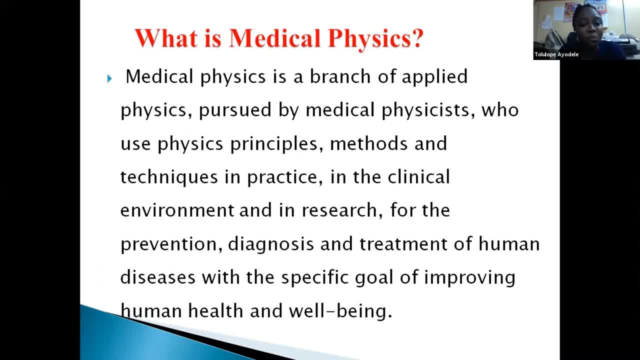 and is pursued by medical physicists. We use physics principles, the methods, the techniques and in a clinical environment in research for the purpose of preventing diseases, for the purpose of diagnosis and treatment of human disease and with an overall goal of human health and wellbeing. 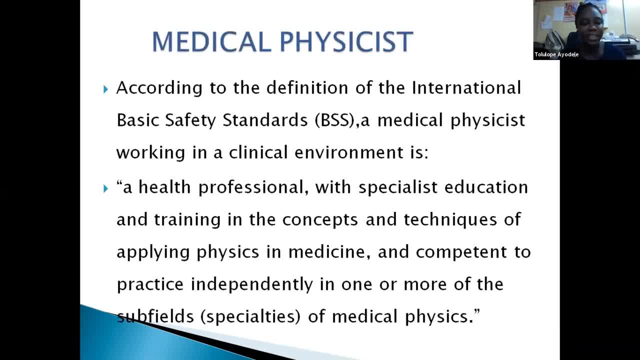 So a medical physicist is defined as the health professional with specialist education and training in the concepts and techniques of applying physics. We apply physics in medicine. Of course, the medical physicist should be competent enough to practice independently in any of the subfields, be it radiation therapy, radiation oncology. 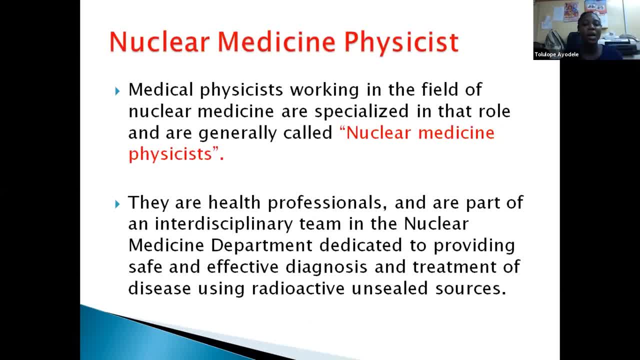 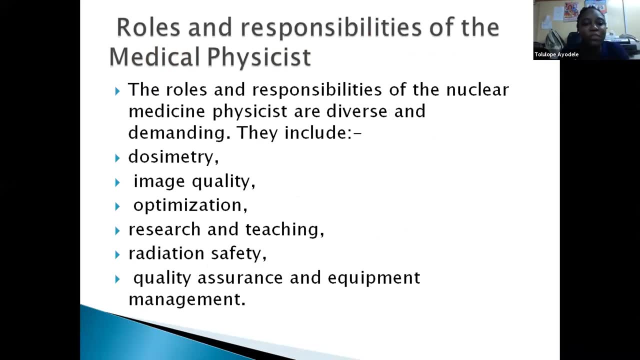 radiology or nuclear medicine. So a nuclear medicine physicist works in a nuclear medicine. the name a medical physicist that works in a nuclear medicine department is a nuclear medicine, is a nuclear physicist. And let's look at the roles of a medical physicists. 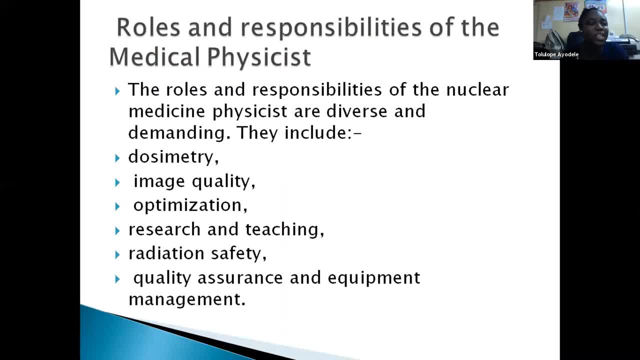 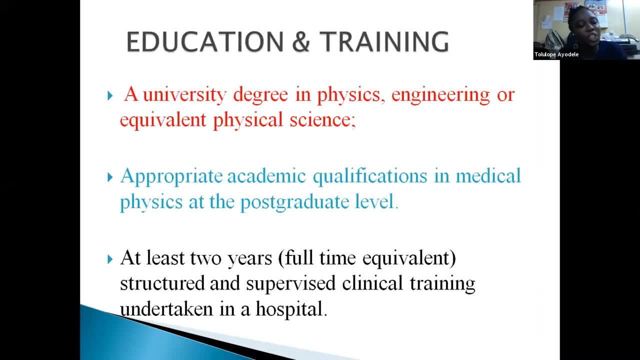 in general, We have. you can see, we have the dosimetry, image and optimization radiation safety. For the education and training of a medical physicist, it involves a university degree in physics, engineering or physical science. Though we have the 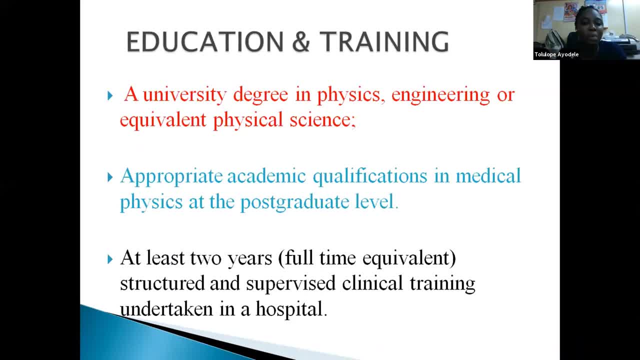 for the different countries have their requirements for this. So we have an appropriate academic qualification at the prograduate level, be it MSc and a PhD, And for one to be qualified as a clinically qualified medical physicist, it has to be well-structured and supervised. 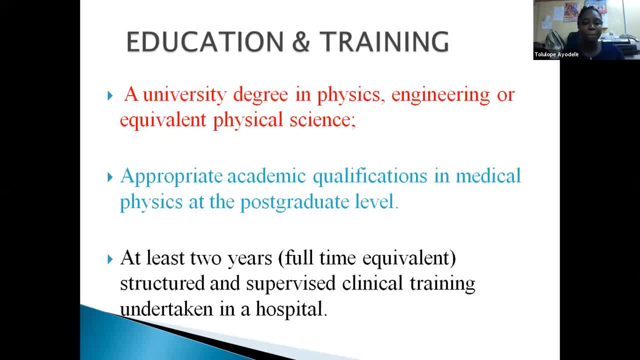 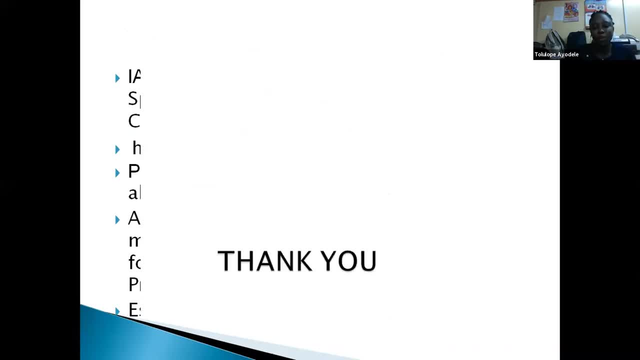 under a clinical, under a clinical training, And that has to be undertaken in an hospital. Thank you All right. thank you very much, Mark, for the lecture. That was a very good presentation. If you have questions, please, you can drop them. 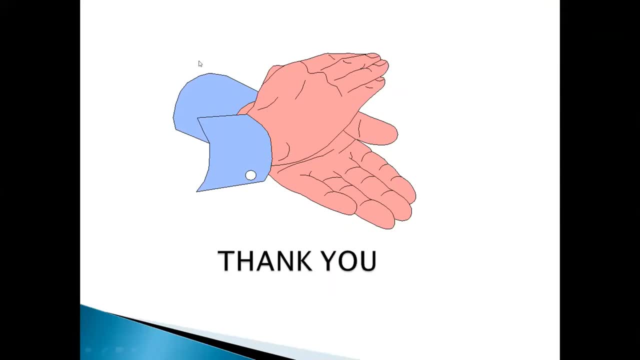 in the comments section of this webinar And we will be happy to answer any questions that you may have. Thank you very much, Mark, for the lecture. That was a very good presentation.